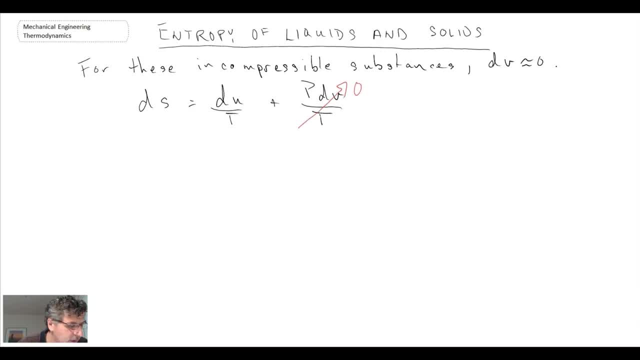 away, so the second term from our equation disappears. The other thing that we can do for the internal energy: we can make a substitution, in terms of our definition, that we had for the internal energy in terms of the specific heat at constant volume. 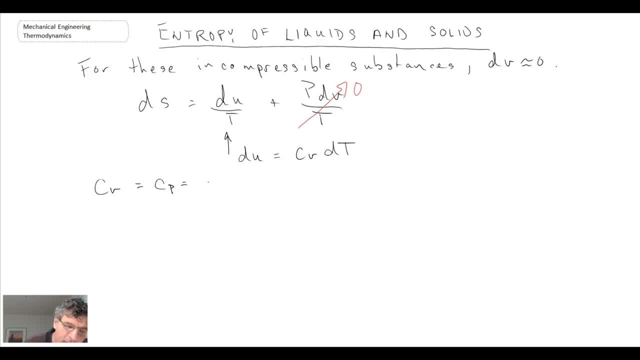 Now, one thing that we'll say about specific heats, for both liquids and solids, is the specific heat at constant pressure and constant volume we will assume to be the same. Now, this is an approximation. it's a better approximation for solids than it is for a. 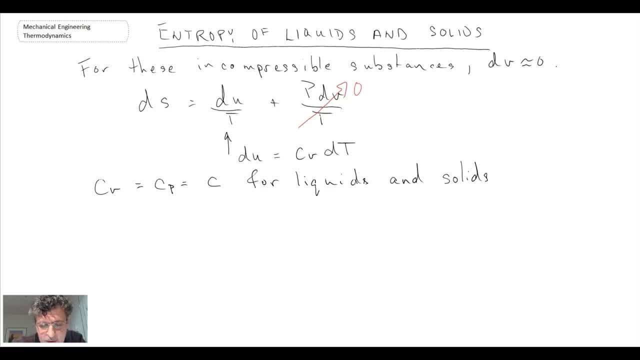 liquid because, for example, if you take water and you heat it, it will undergo volumetric expansion, so it will change a small amount. However, what we will do is we will assume that that change is negligible for our purposes and consequently, we will consider the specific. 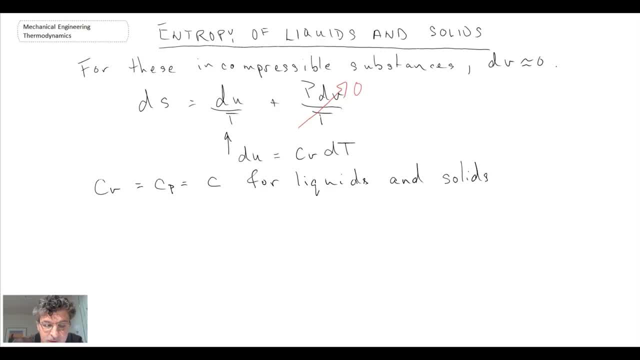 heat at both constant volume and constant pressure, to be the same for both liquids and solids, and with that we can rewrite our equation, the differential form for the entropy, as being specific heat, now not specific, either constant volume or constant pressure, and we get this equation. now what we're going to do is: 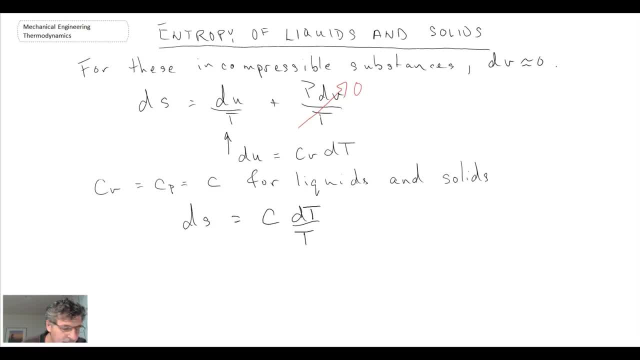 integrate that between two states, the beginning state and an end state, so we get this integral equation. and you'll notice that I've written the specific heat here to be a function of temperature, integrating that equation. and we can integrate it if we assume an average specific heat for our process. 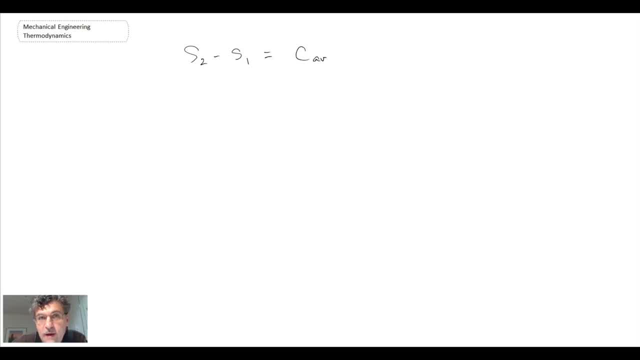 otherwise you need to know how the specific heat will change with temperature for that particular solid or liquid. but if you can assume an average specific heat, that would be the equation that you then use to calculate the change in entropy for that solid or liquid. a final comment about this.